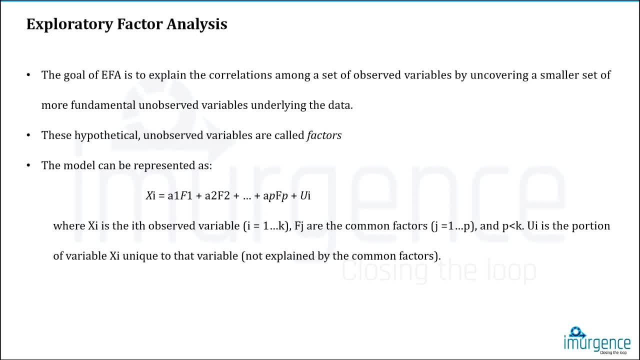 if I can take that as a numerical data right. So number of vowels present in say Mohan, in the word Mohan. So if I say A and O, there are two right: M, O, H, A, N right There are. 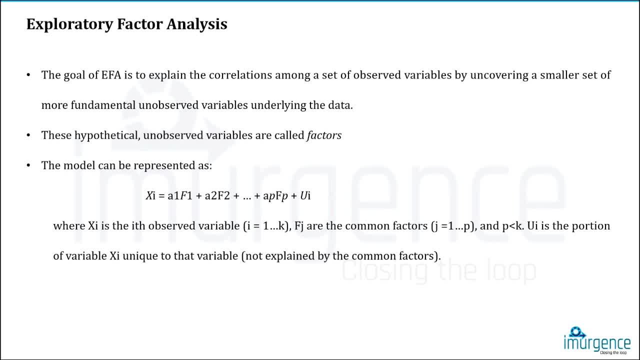 two vowels in my name, right, If I keep on counting these vowels in everybody's name, if I have the data And similarly, if I say that the names will start with a vowel, then I mark a one or a zero And similarly I can do feature extraction from all these set of. 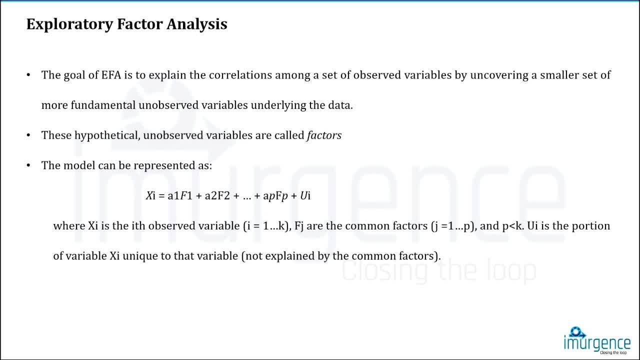 data. Now, these are very small, small things, but if they connect together as a factor, it starts really talking about your dependent variable that, yes, whether this person is a male or female, can be isolated right. So your intention in exploratory factor analysis? 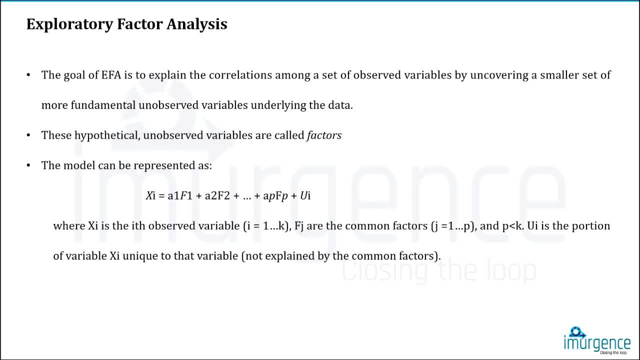 is to understand that hidden part right, And the model is usually represented by the X i is equal to A 1 F 1.. So A 2 F 2 plus dash, dash, dash, plus A P, F, P plus U, i right. 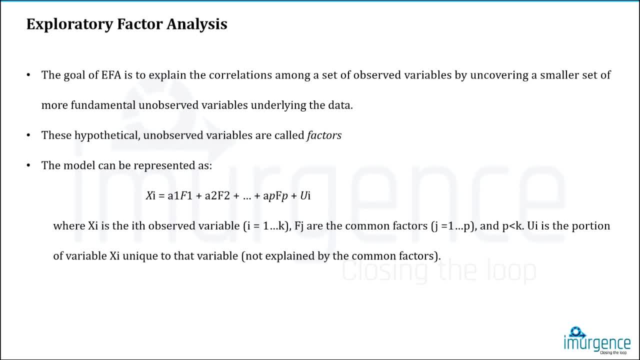 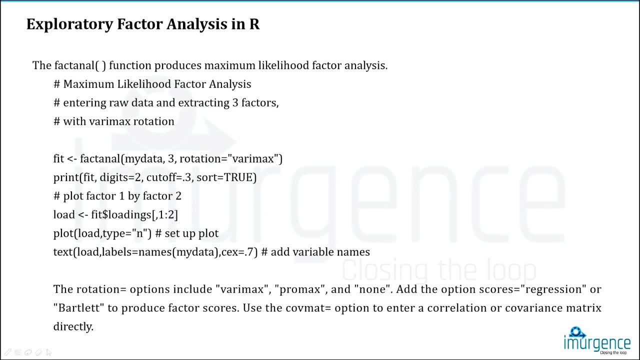 Where U i is the proportion of variable X i unique to that variable not explained by the common factors, And X i is the ith observed variable. F, j are the common factors, So j can start from 1 to P and P has to be less than k, So the fact annal. so it is F A C. 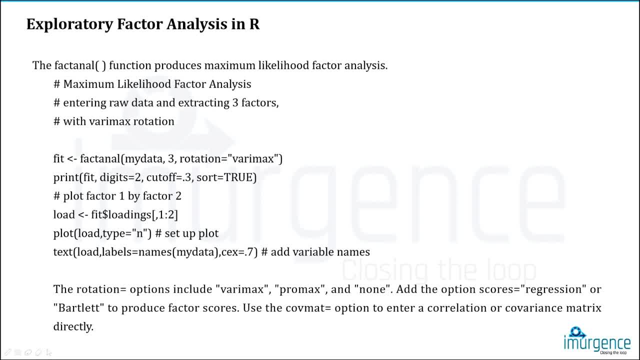 T, A, N, L, That is factor factor analysis function provides maximum likelihood factor analysis. So you have to enter the raw data and you have to specify the number of factors you want. right, So it has the very max rotation. So a typical function call would be like you call the fact. 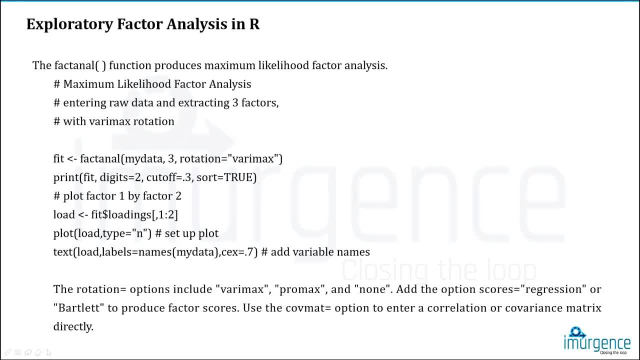 annal function: pass the first object as the data, the number of factors as the second one, the rotation. you have to specify whether it is very max or not- And then you get the algorithm to run on this data and you can save it in an object of your own preferred. 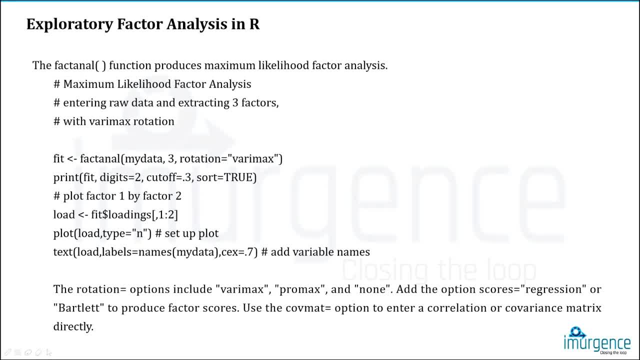 name. You can check the same thing as what you did in the previous case You can check. So principal component analysis and factor analysis somewhere comes very close to each other because we are dealing with dimensions over here. So the loadings can be checked. 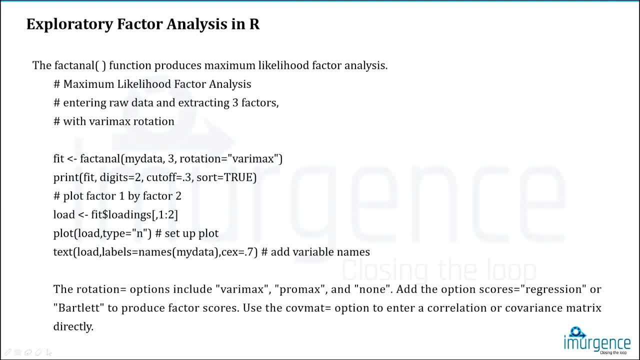 the plots can be done in the same way as what you had done over there, right? So the rotation includes very max pro max, none, right? And there are other options, like when you want to do scoring, you can do a regression. 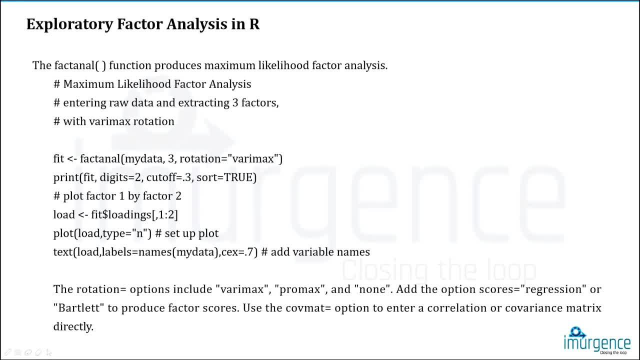 or a barlet to produce the number of factors. So the number of factors, right, You can produce factor scores. you can use the covariance covmat option to enter a correlation or a covariance preference. right, so you can say that. so in the previous case you had said: 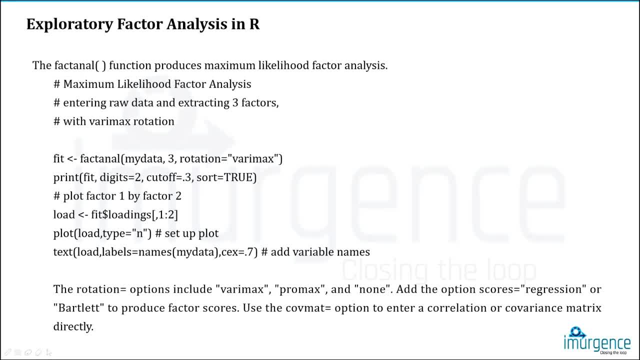 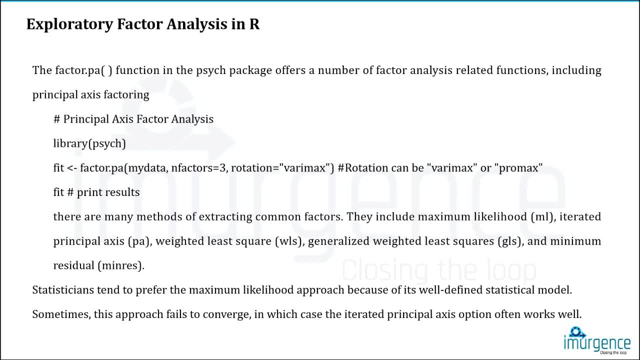 cor is equal to true or cor is equal to false. which did that? in this case, you can specify covmat whether it is correlation or covariance matrix. right the fact? factorpa function, which is part of the site package, offers a number of factor analysis related functions, including principal axis factoring. so you have factorpa. that's a. 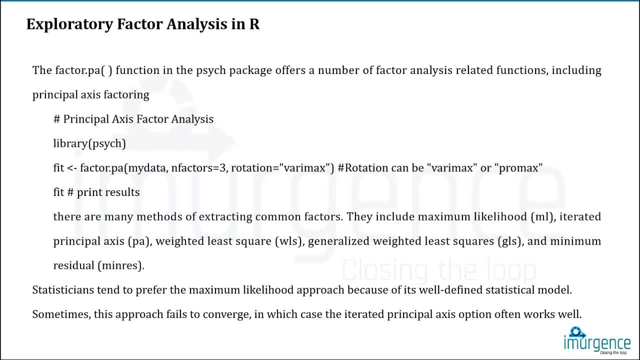 function. again, you have to pass the data, you have to pass a number of factors, you have to specify the rotation method which you want, which can be varimax or promax, and then you can. it includes the maximum likelihood iterated principal axis, right? so when you come to the factor extraction, 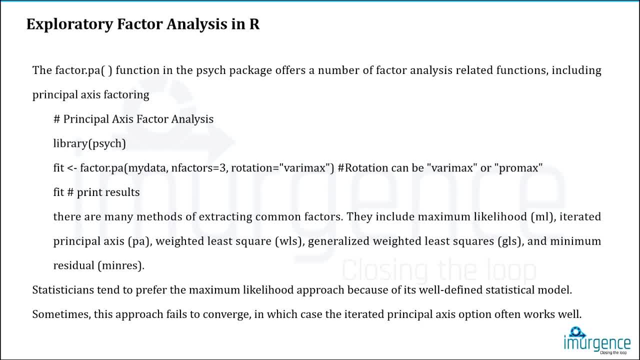 method. there are these methods which are like the weighted least squares, generalized weighted least squares and the minimum residuals, that is, min res. all these options are available. now statisticians tend to prefer the MLA approach because it is well defined from statistical perspective. so, maximum likelihood estimates: the generalized weighted least squares. right, the weighted least squares. 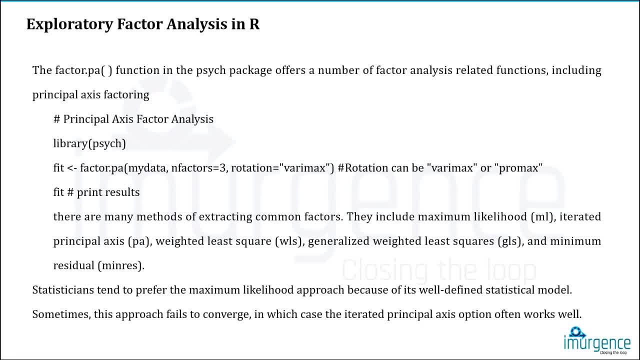 is somewhere coming close to the linear and logistic regression concepts and becomes more relevant to statisticians. sometimes these approaches fail to converge, in which case the iterated principal axis option is the one which works well most of the time. so if these don't work for you, then you have to pass the data, and then you have to pass the data to the. 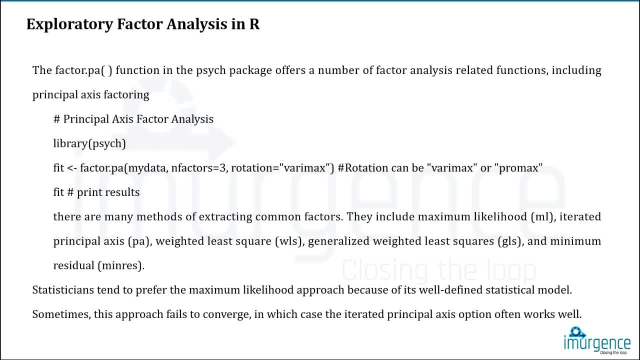 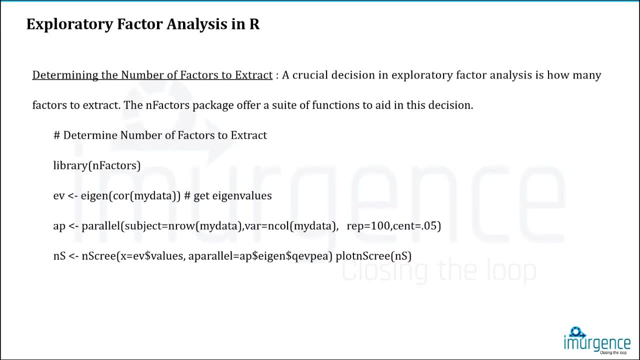 principal axis option, which usually works most of the time right. so sometimes data might say error, couldn't find these many factors and all those things. so that's the time when you can try, as a last option, the iterated principal axis. now, when you're doing this exploratory factor analysis, you 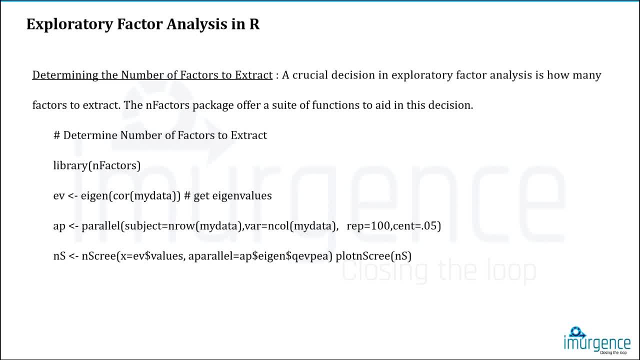 have to determine the number of factors to extract. so in this case, we said in the previous what you can see on the screen, that three was mentioned, or how did you arrive at that three? now you have to get that decision. you have a different function, which is called as n factors, which offers a suit. 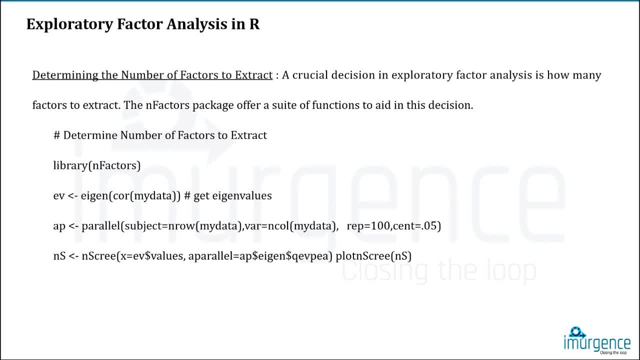 of function to aid you in this decision. so you have to just load that package n factors and then you will use the IGN values, right? so you have to call the IGN function. you have to pass the correlation of my data. so you're passing the correlation grid, the whole matrix, and you're. 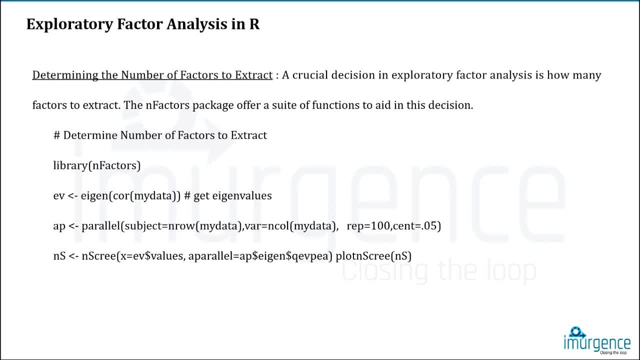 going to compute the distance between these, that is, the IGN direct distance between these. and then you are trying to use a parallel function wherein you are saying something like this: is equal to n row, my data, number of rows. the variance is equal to number of columns, my data, and replicate 100 times percentage is equal to 0.05. and then you say n scree, in which 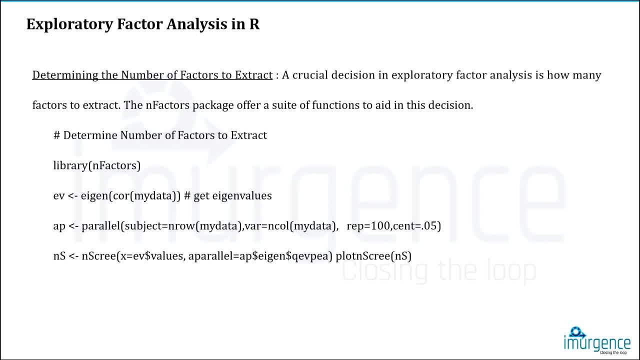 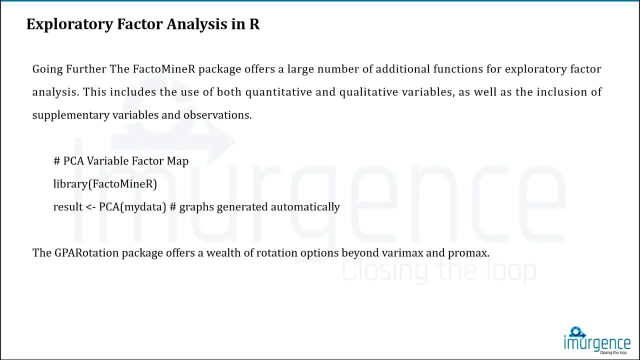 you're passing the IGN values which you had collected in the previous case, the matrix, parallelized matrix that you're going to pass and you're just going to plot it. first, there is a factor mine r package which offers a large number of additional functions for exploratory factor. 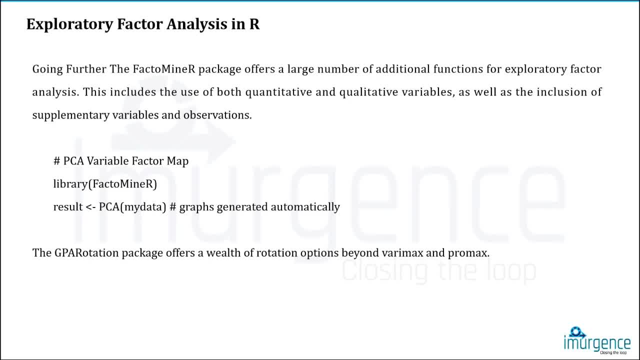 analysis. this includes use of both the method and the method of the method, of the method of the method, qualitative and quantitative variables. right, so you have to load that package, factor mine r, and you can directly run a pca on the data without specifying anything and it will automatically. 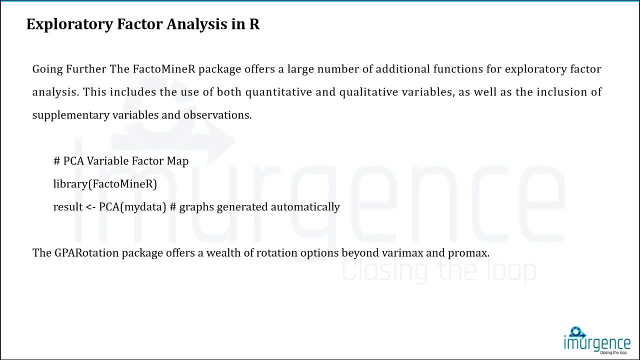 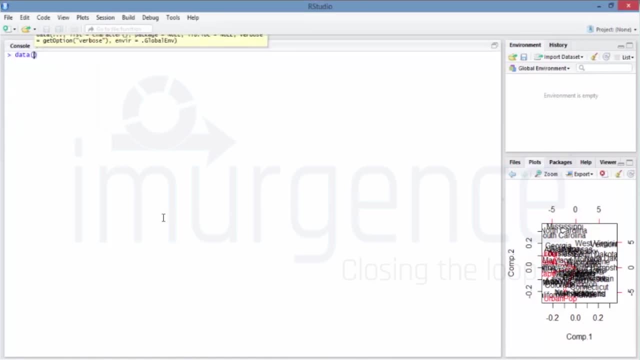 generate the whole set of results for you and the object which you specify. the gpa rotation package offers a wealth of rotation options which goes beyond varimax and promax computations. so we'll see the application of factor analysis over here. so we'll load the data. so again we're. 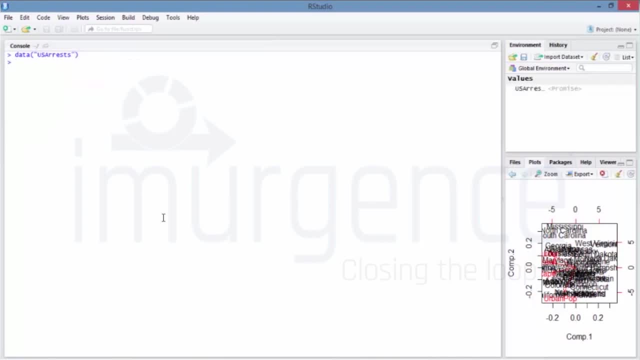 going to use the same old data, usa arrest data. we're going to save that in usa location, usa list. it sets the data and then we'll install the package n factors. so i have already got that installed, i guess, so i'll just check it whether i have it in factors. yes, it's there, so i'm just 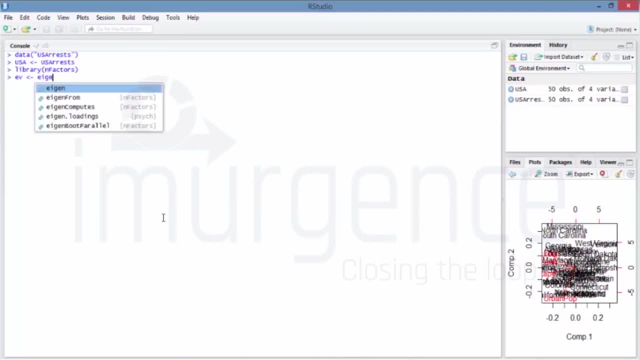 loading that package you will use a variable name in which you want to store the output of the IGN values which you are going to compute. so we're going to say IGN correlation function and in that you're going to pass the usa data right, so that will be stored. 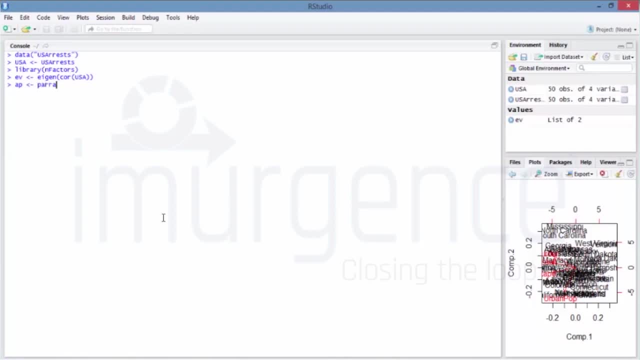 in ev and then you're saying ap. you're creating one more object where you're saying parallel, in that you're passing: subject is equal to number of rows of usa, so it will be computed at runtime, and var is equal to number of column of usa and spelling is parallel. 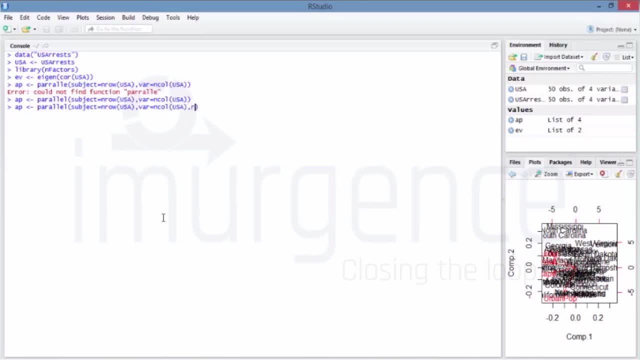 okay, so these two things are done. uh, i guess we have to add one more parameter after the us. it's replicate is equal to 100 and sent is equal to 0.5, right, and then you're going to say n, the capital s with this, because we're going to do a scree plot. so i'm saying n. 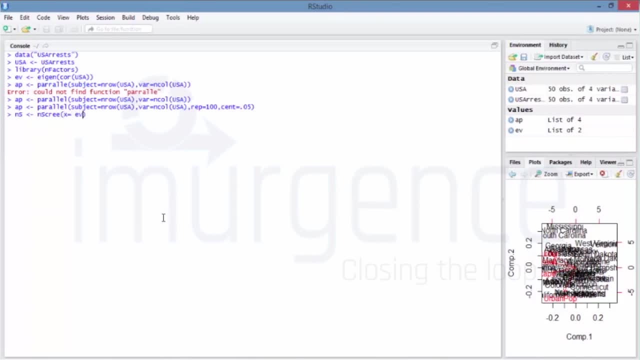 scree in which you're going to say: x is equal to the IGN values which you have computed, which is saved in the ev object, and then the a parallel is equal to ap, dollar, IGN, dollar, q, e, e, p, a, and then just do an enter and you say plot. 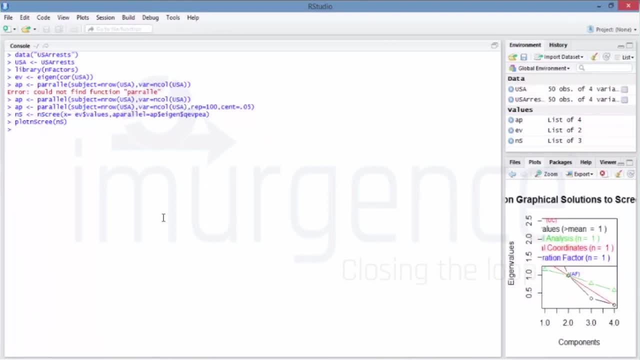 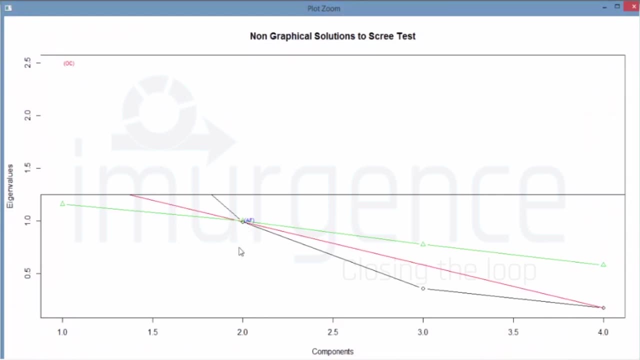 scree and in that you're going to pass this new object, you'll be getting somewhere. this is cluttered, but this is how it is. it's. it's basically to understand how many number of clusters, how many number of factors you should be selecting what is optimized. so usually see where these green and the black line converge and 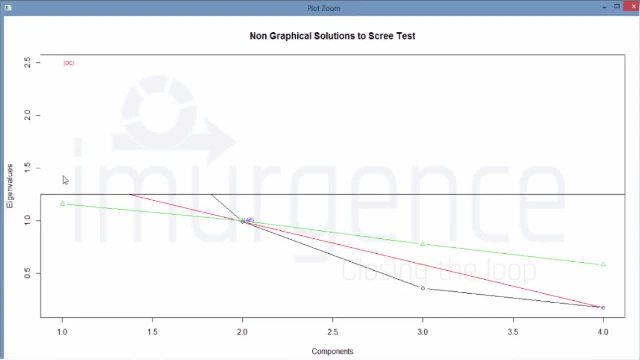 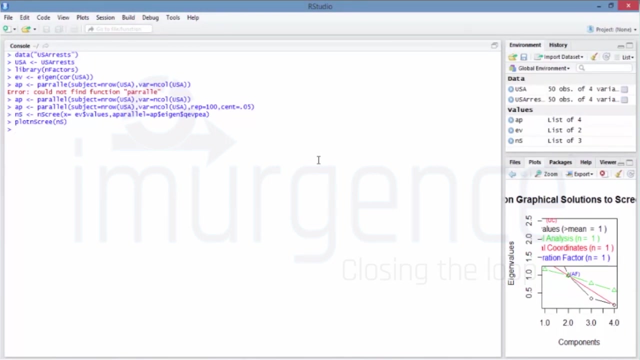 the number of greens which are there before this. so obviously this is cut off over here, but this plot should be till here, and obviously there is only one which is before that. so the optimized k, that is, number factors over here, looks as if one, but still because we want to show it, so we'll. 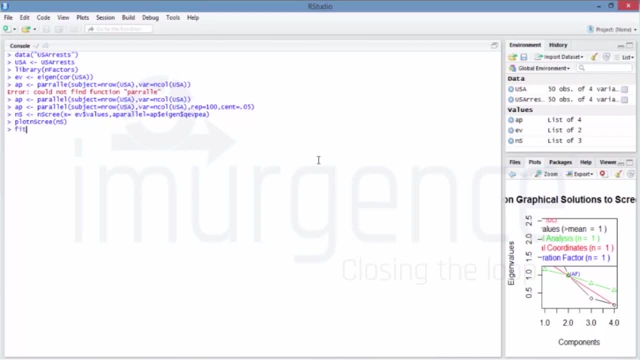 go beyond that right. so we'll say: fit 11, allocation sign and fact annul. that's the functionality we're using usa comma 1, because we found that there was only one optimized factor. count rotation is equal to vary max, right, you can say print of: 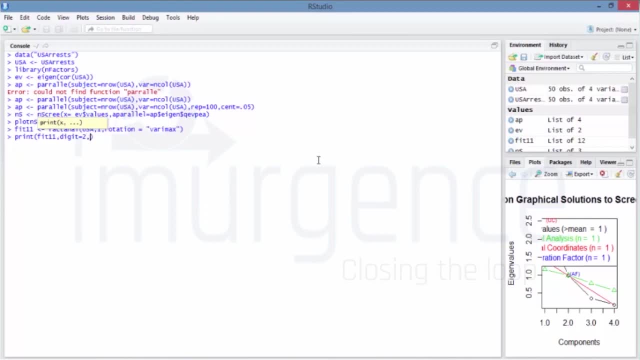 you can also call this fit11 comma. digits is equal to 2 and cut off the cutoff value, beyond which you are saying that the component should be part, is 0.3. that is, you are specifying sort is equal to true. okay, so these are the various columns in the data you said to create one factor. 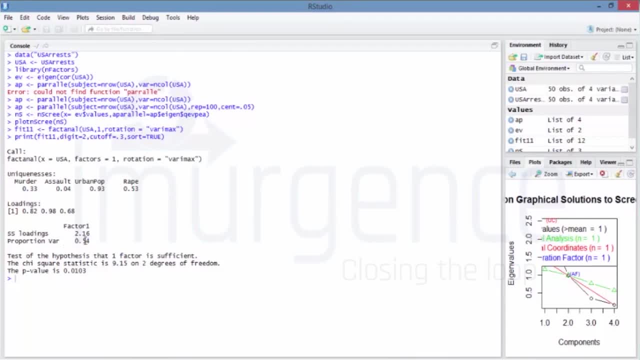 only one factor for accidentally creating a new filter factor has been created: the sum of square of loading and the variation. The test of the hypothesis is that one factor is sufficient. that is the hypothesis which is running over here. the chi-square statistics is 9.15, which is very high, and the corresponding 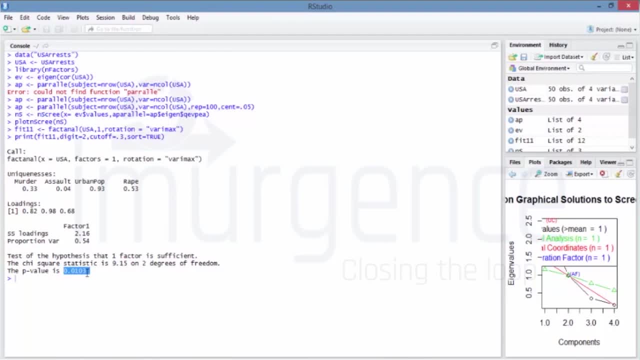 p-value is 0.01, which obviously is very low as compared to the standard cut-off p-value, which is a 0.05.. So obviously what it says is that this is significant and this makes sense. Now you can plot factor 1 by factor 2 also, so you can say a load allocation fit $11 loadings. 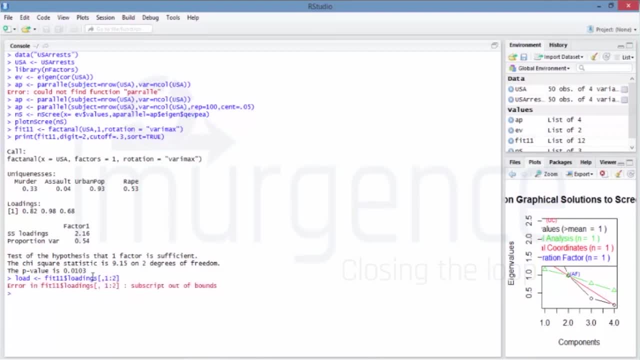 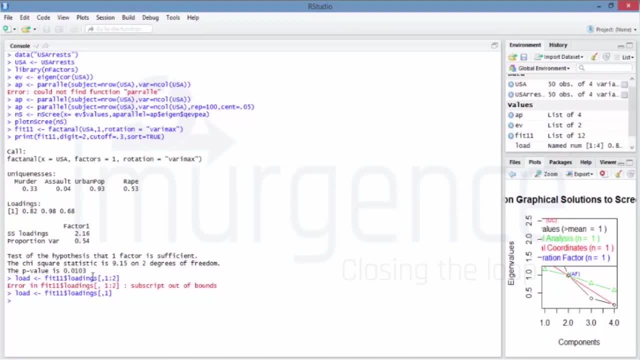 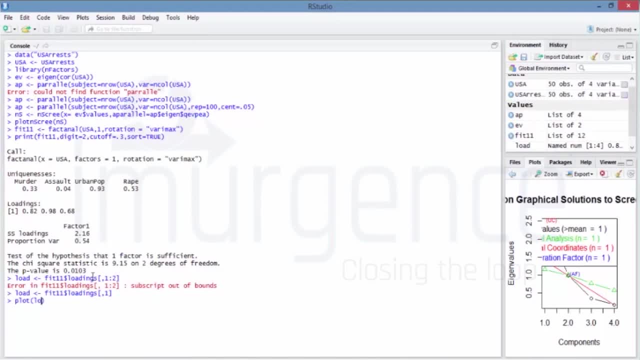 So you can say: 1, plot load type is equal to n and text load. now we cannot do plot factor 1 by factor 2 because we just have one factor in our data, right for left, for fit 11, we passed fact and the USA comma 1, so we 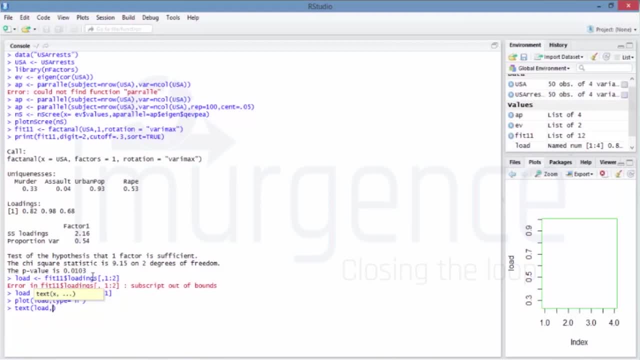 ideally told the algorithm to create one factor. now, when we are saying that, plot factor 1 by factor 2, so it won't come out because we haven't created that. still, as you can see on the screen, we just process the algorithm. so labels is equal to names, USA comma 3x is equal to 0.7. let's show that's where they're. 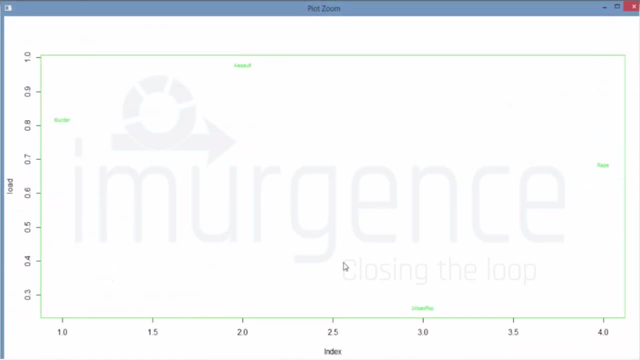 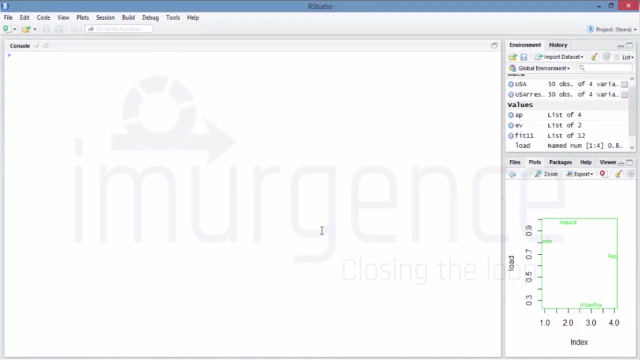 standing murder, assault, rape, urban probe. but you just have one factor, you don't have two. that's why it is coming like that and the index is just coming because of absence of the other factor. okay, so, as you can see on your screen, you already have made and call that. you're. 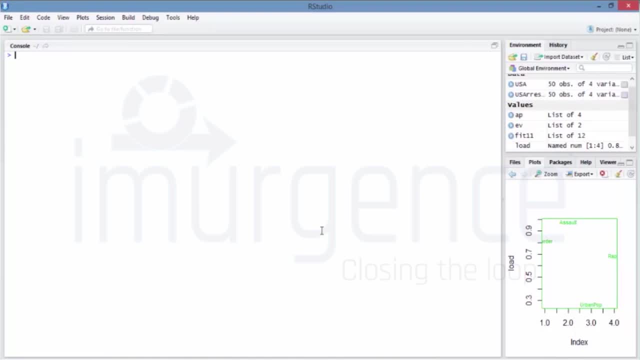 going to take on the one factors, because the number of green boxes before the intersection of the black and the green is only one. so you have said the optimized number of factors is one and correspondingly also you saw that when you do did this, the hypothesis test said that your p-value is 0.01 approximately. 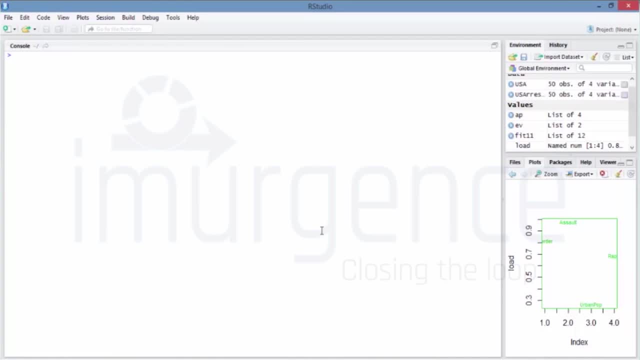 which is less than 0.05, which is significant, right? so that makes sense. okay, so now we are going to take a look at the hypothesis test that your p-value is 0.01 approximately, which is less than 0.05, which is significant, right? so that makes sense. 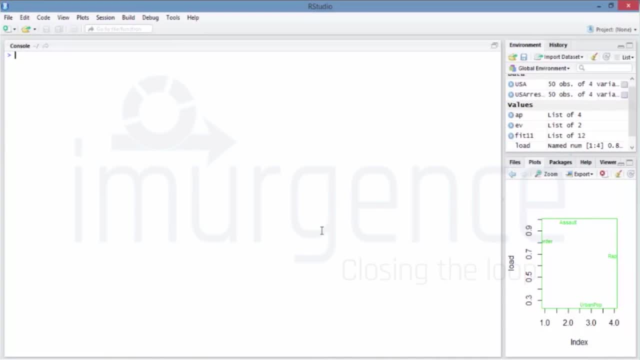 right and again. an output of the same which we saw on the screen when you're doing it over here is shown. over here, the chi-square fit statistics is very small. this indicates that the hypothesis of perfect model fit is rejected and the alternate hypothesis is selected. so what's the difference between a PCA and? 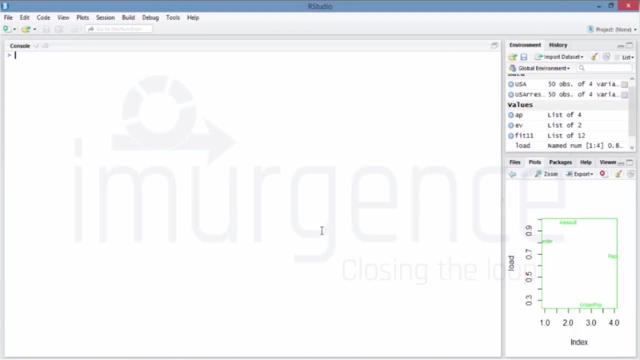 EFA. the PCA is useful for data reduction method that can replace an A's number of correlated variables, which is called as multi-collinearity, with a smaller number of unto-coincidental variables- uncorrelated variables- simplifying the analysis, Whereas the exploratory factor analysis contains a broad range of methods for identifying. 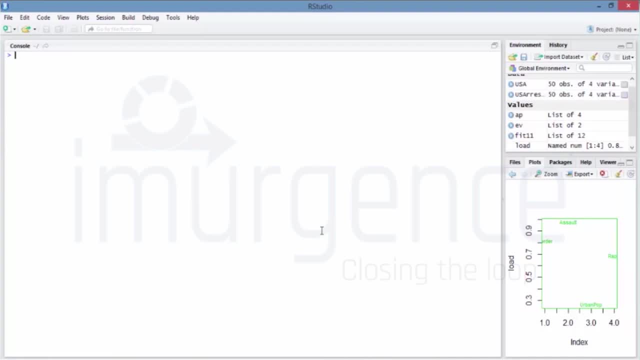 latent variables or unobserved constructs that may underlie a set of observed or manifest variables. Again, you need to understand the perspective. Now, exploratory factor analysis is more often used when you're doing research, when you're distributing survey forms, For example.